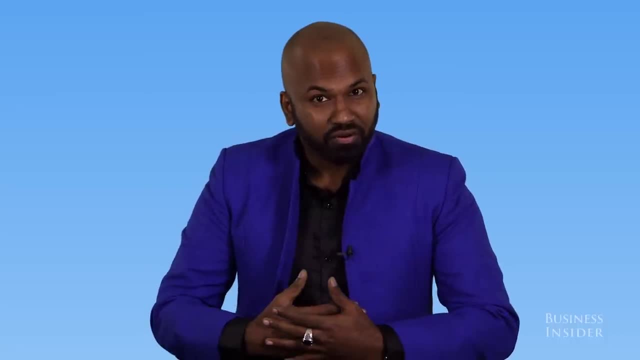 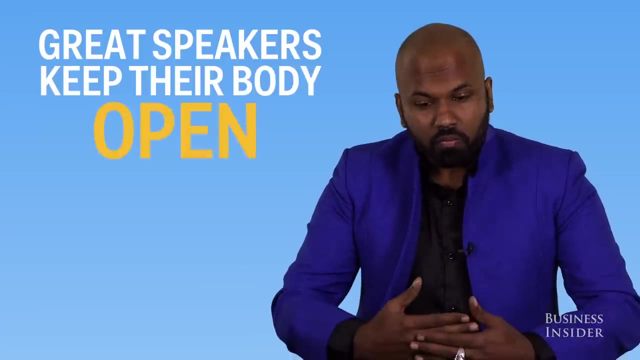 sometimes fold their hands, bring their hands in front of them, And that's a sign of nervousness. Great speakers keep their body open, So there is no barrier between you and me. Raise your hand. if you have an emotional mother, Let me see. 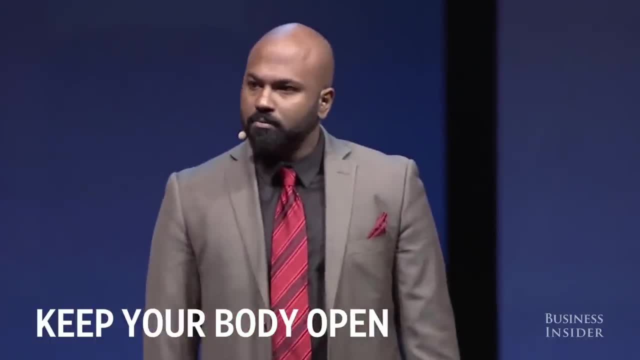 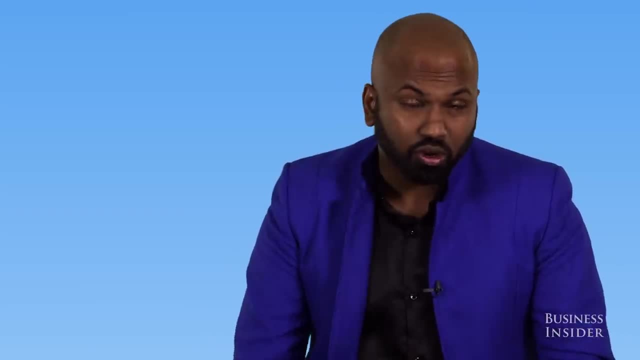 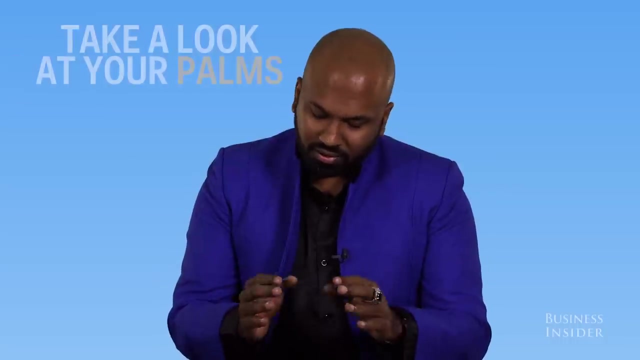 Put them all together, You get mama, And something that, when you're starting out, you got to be very conscious about is keep your body open. Here's tip number two: Have your palms open. Do this exercise with me. Take a look at your palms, Turn them around. Take a look at the inside of your palms again. 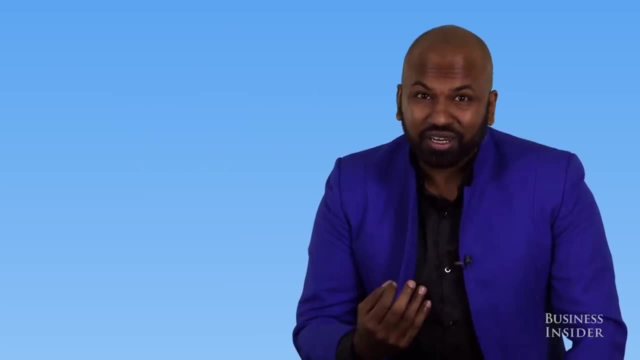 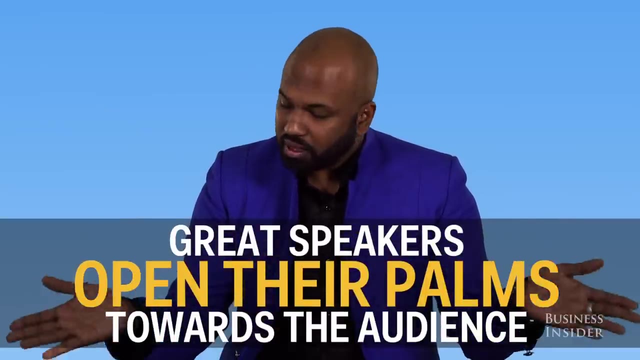 What side relaxes your eye? If you're looking at the inside of your palms, what side relaxes your eye If you really concentrate? when you look at the inside of your palm, your eye relaxes, And a lot of great speakers they open their palms towards the audience, showing a more openness. 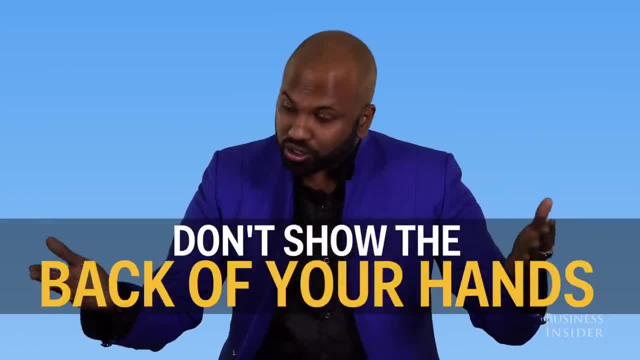 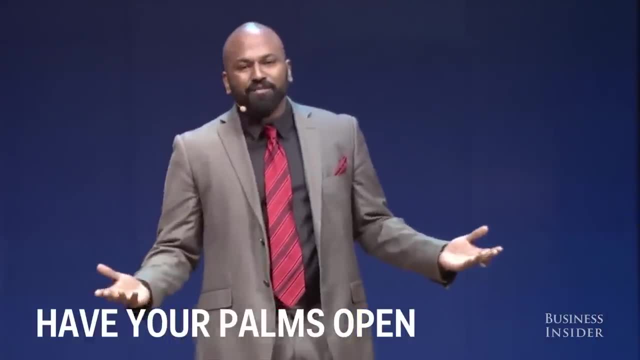 And that allows the audience to connect with the speaker better as opposed to showing the back of your hand. Ladies and gentlemen, today I'm a dreamer, I'm a speaker And I learned the unfailing quality of unconditional love from my wife. 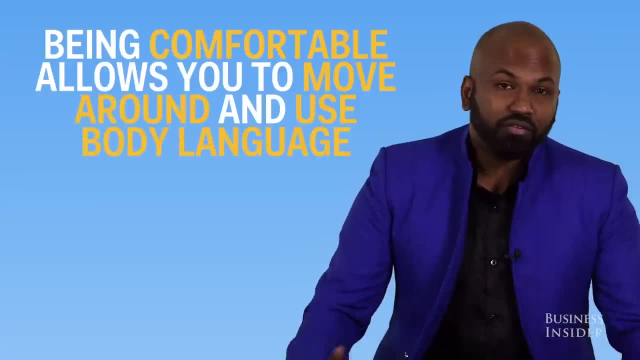 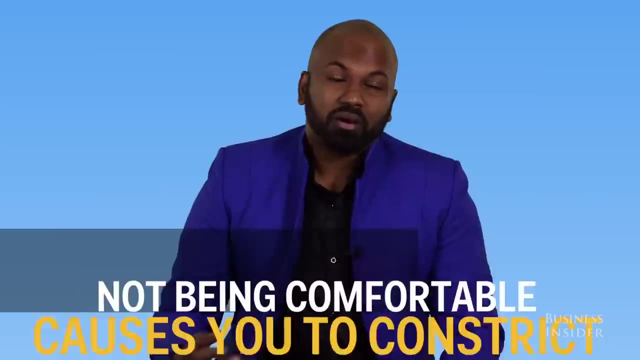 Number three: get comfortable with the stage. When you're comfortable on the stage that you're speaking on, your body is freer to move about, use body language. But if you're not comfortable with that stage and if you feel foreign on that stage, 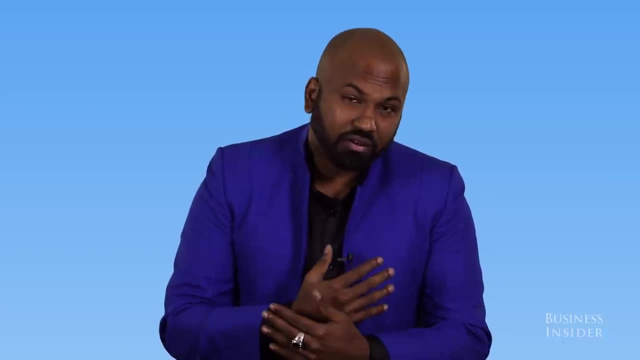 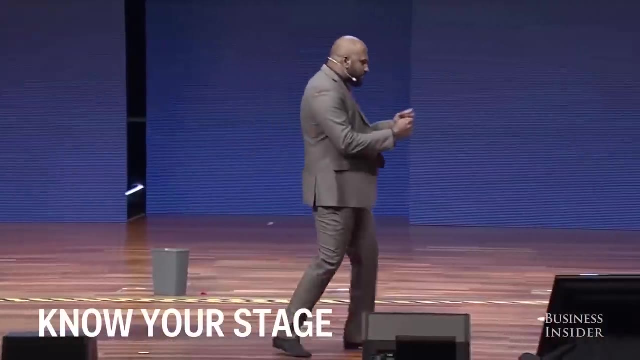 what happens is your body language starts to constrict and you start to cover your body up. And when a son sees a mother cry tears of shame, that's a life-changing moment. She looked at me and said, son, I want you to be a better man. 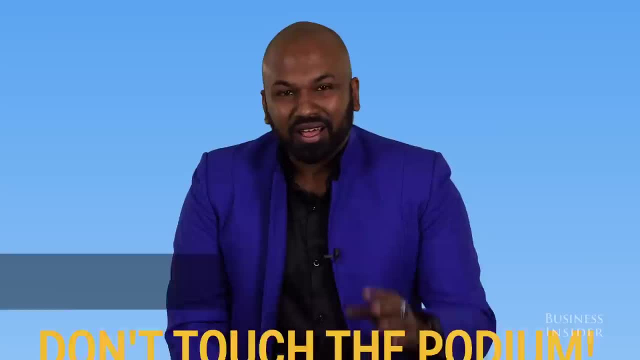 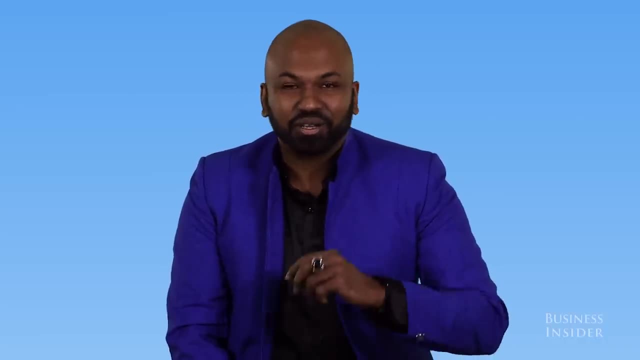 Number four: get comfortable with the stage. Whatever you do, don't touch the podium. As soon as you do that, you're going to be leaning on it, you're going to be shaking that podium and you will be doing all sorts. 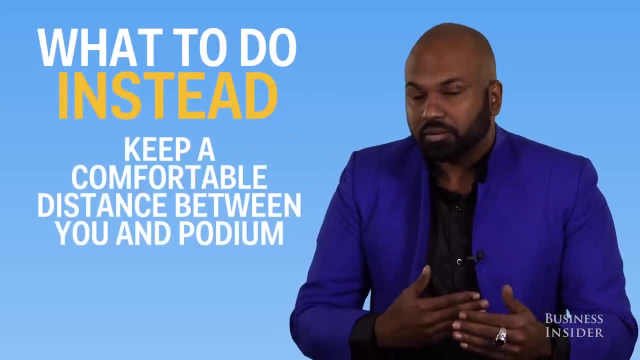 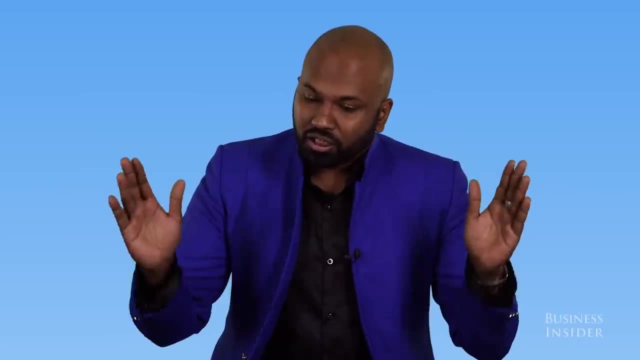 of things on the podium. So what you do is you keep a comfortable distance between you and the podium. You can keep your notes on it, but you can use your hands to gesture. Don't rest your hands on the podium. So keep a distance and you can gesture, use body. language as you want, from a little distance from the podium.